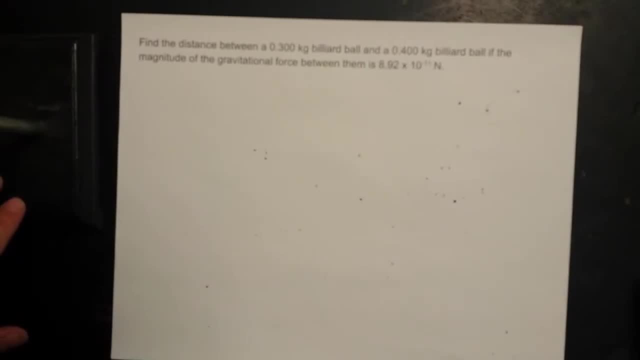 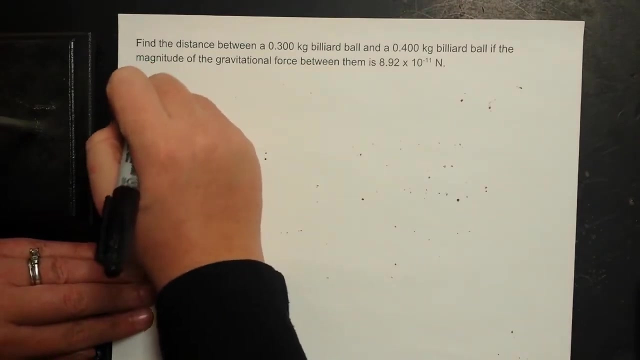 In this practice problem we're going to calculate the distance between two billiard balls, given their masses and the gravitational force between the two of them, and I'm sorry it's out of focus. Alright, so we've got two billiard balls. Mass of my first billiard ball is 0.3 kilograms. Mass of my second billiard. 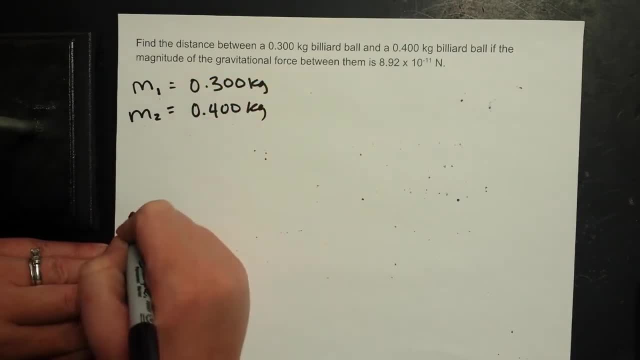 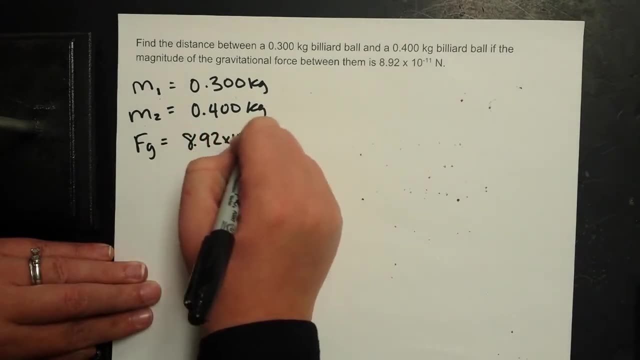 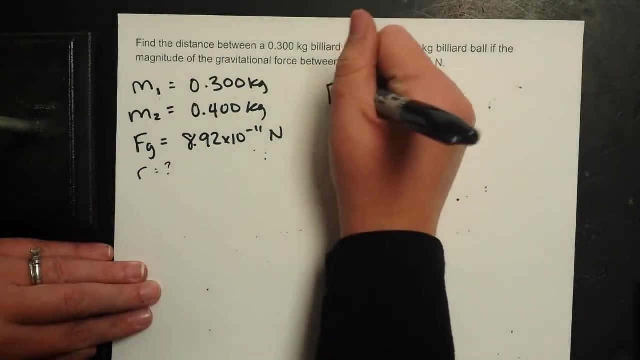 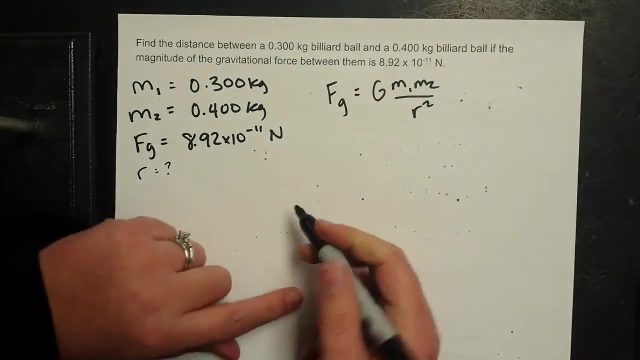 ball is 0.4 kilograms. My gravitational force between the two of them is 8.92 times 10 to the negative 11th Newtons, and I'm looking for the distance between them Alright. so remember, FG is equal to big G, M1, M2 over R squared, I can say the: 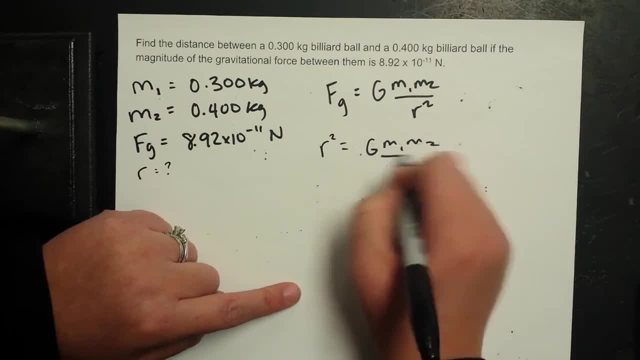 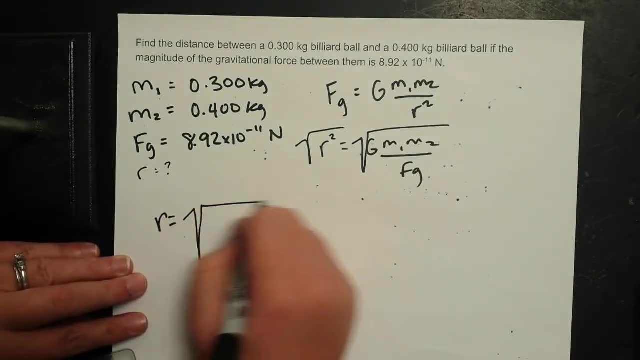 R squared, then is big G M1 M2 over R squared, Big G M1 M2 over FG, and the square root both sides- So now I get the distance- is the square root of the constant of universal gravitation times, the product of both. 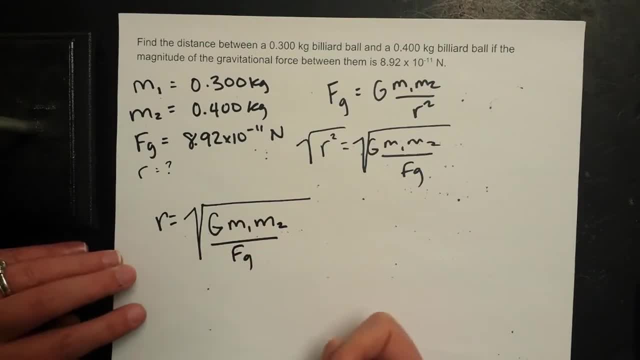 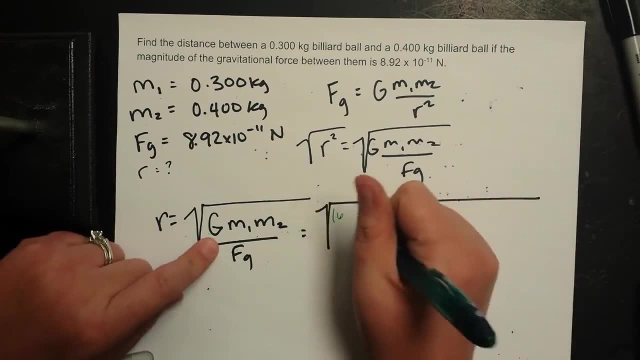 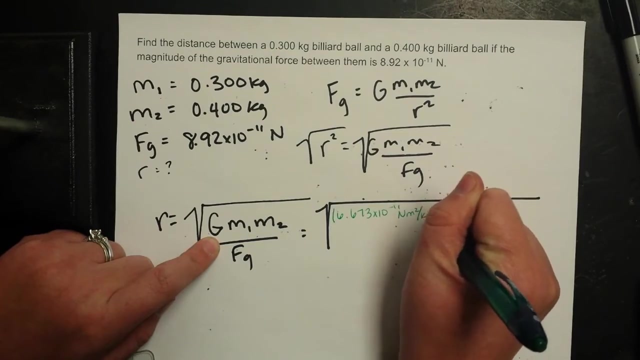 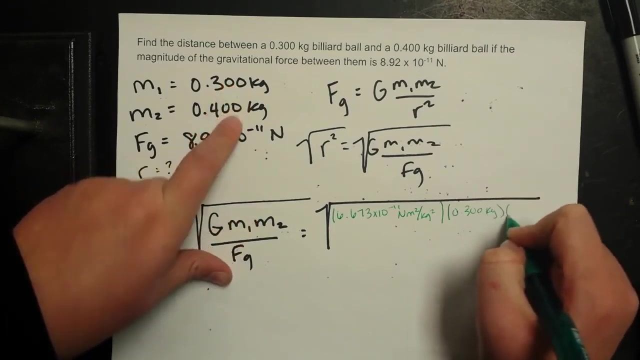 masses all divided by the gravitational force. Plug in what I know and I'm going to use pin this time. So big G is 6.673 times 10 to the negative 11th Newton meters squared per second. Big G is 6.673 per kilogram squared times 0.3 kilograms times 0.4 kilograms all divided. 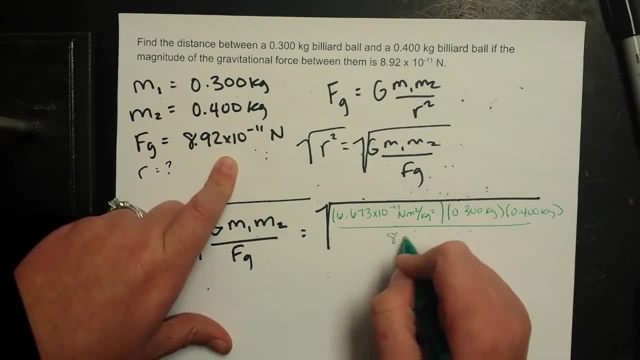 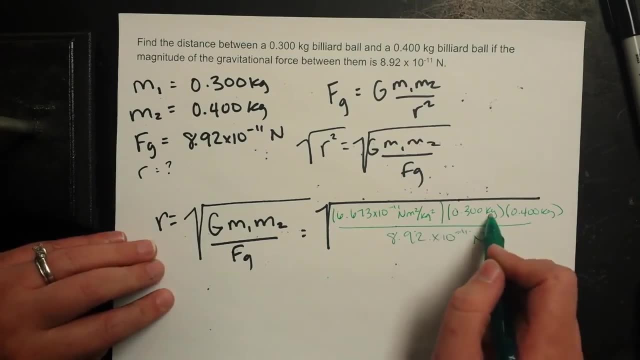 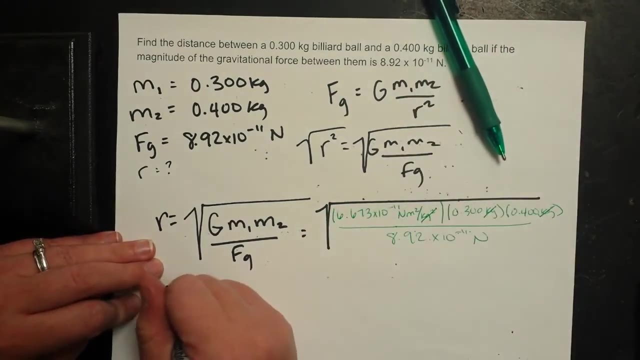 by my gravitational force, which is 8.92 times 10 to the negative 11th Newtons. To solve my numerator, I do see that this kilogram times kilogram will cancel out my kilogram squared, So I got R then is equal to something with a Newton meter squared all over 8.92 times 10 to the 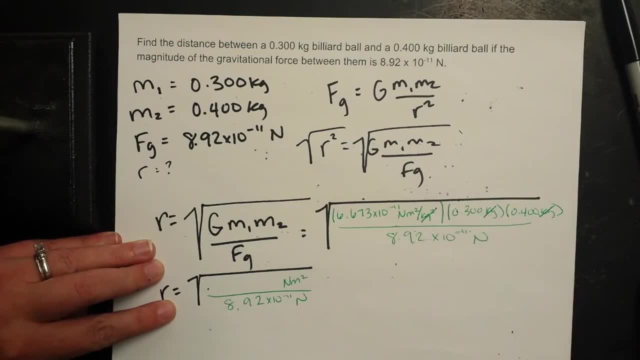 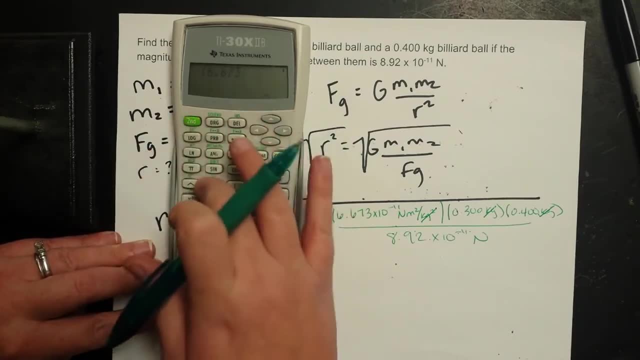 negative 11th Newtons. Alright, so I go ahead and multiply across the top. I'm going to have in my numerator 6.673 times 10 to the negative 11 times 0.3 times 0.4.. Oops, I'm. 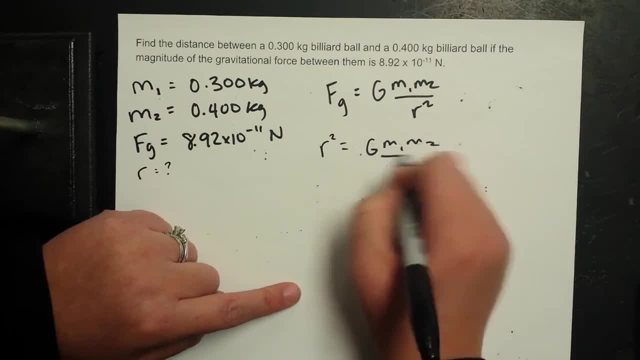 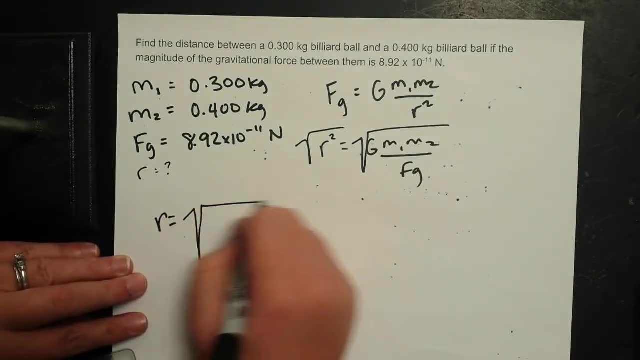 R squared, then is big G M1 M2 over R squared, Big G M1 M2 over FG, and the square root both sides- So now I get the distance- is the square root of the constant of universal gravitation times, the product of both. 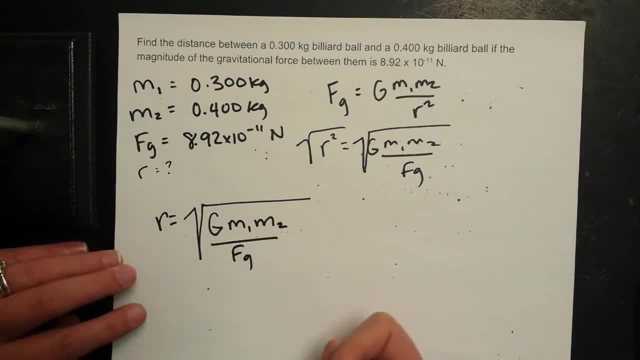 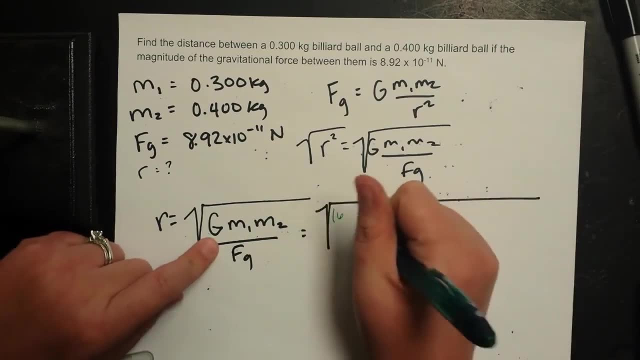 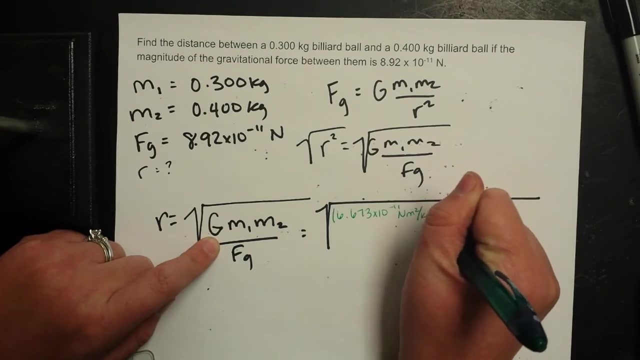 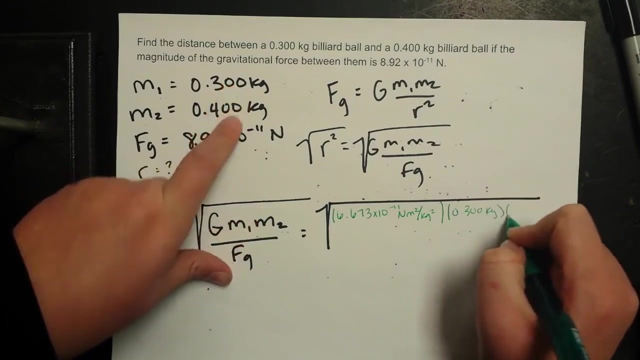 masses all divided by the gravitational force. Plug in what I know and I'm going to use pin this time. So big G is 6.673 times 10 to the negative 11th Newton meters squared per second. And I got C X squared per kilogram squared times 0.3 kilograms times 0.4 kilograms. 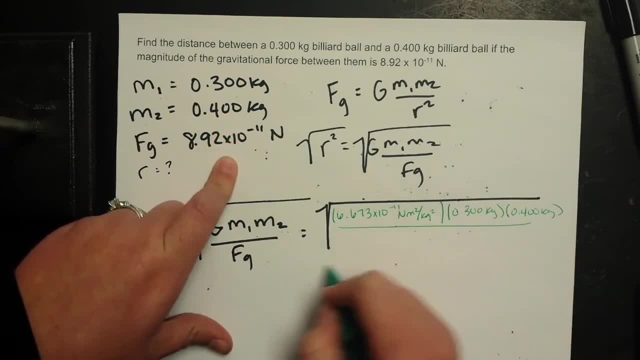 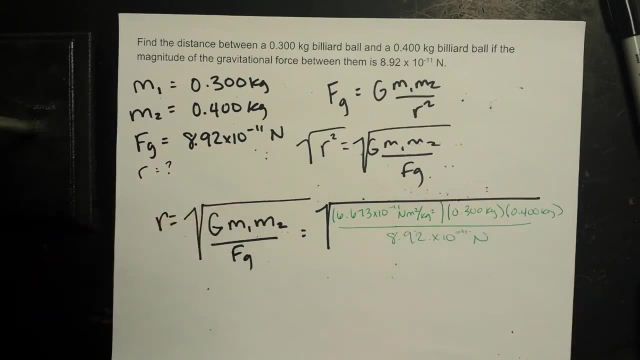 OK, all divided by my gravitational force, which is 8.92 times 10 to the negative 11th Newtons. OK, to solve my numerator. I do see that this kilogram times kilogram will cancel out my kilogram squared. OK, so I got. 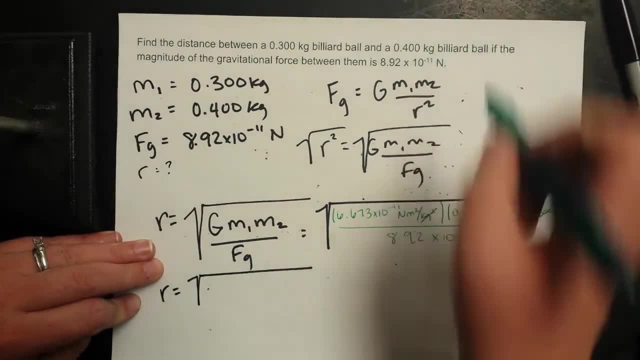 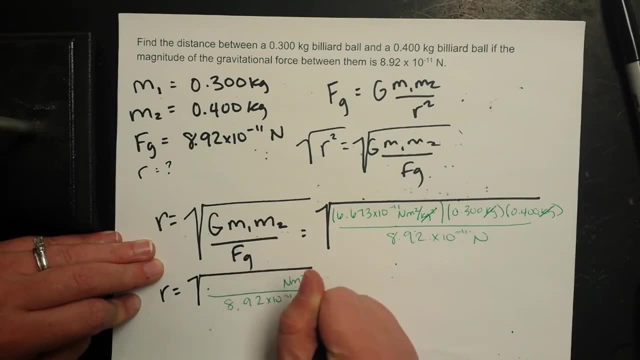 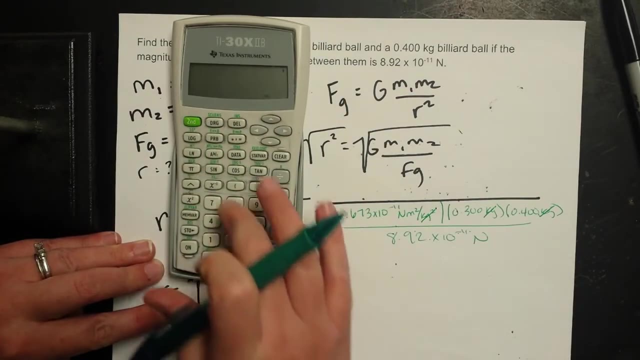 R, then, is equal to something with a Newton meter squared all over 8.92 times 10 to the negative 11th Newtons. Alright, if I go ahead and multiply across the top, I'm going to have in my numerator 6.673 times 10 to the negative 11 times 0.3 times 0.4.. 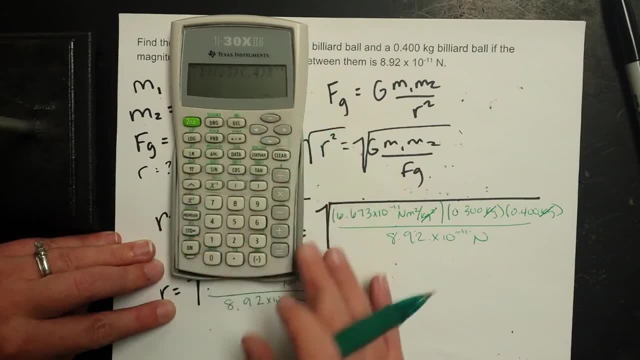 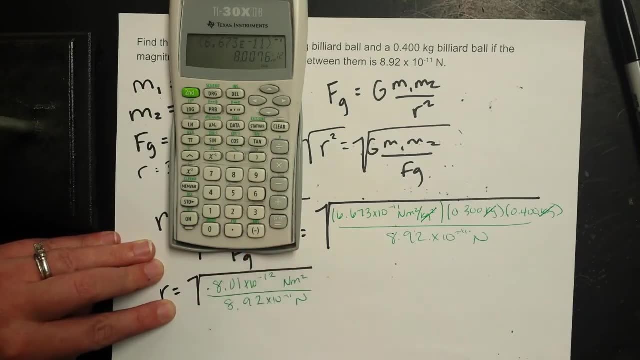 Oops, plus 0. I'm not going to confuse you guys with that, so we'll just delete that, Alright, and we get 8.01 times 10 to the negative 12th. Okay, Alright, I can take this numerator and divide it by my denominator. 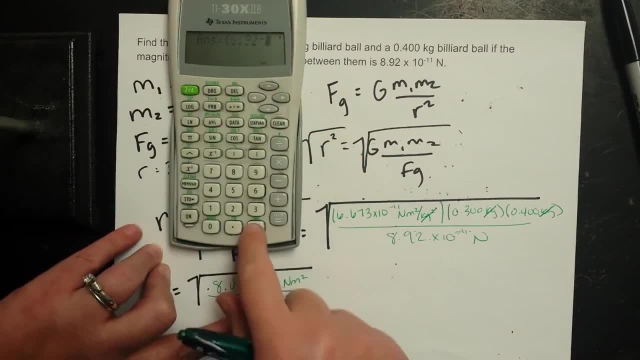 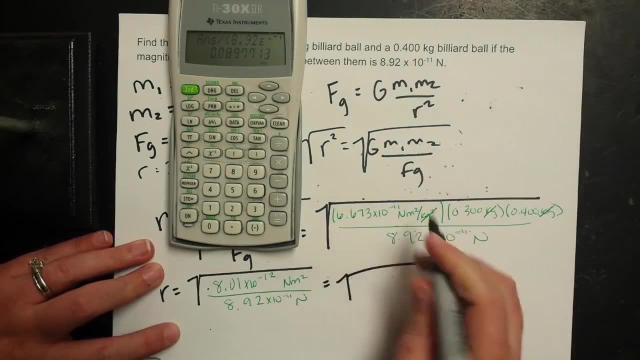 So I divide it by 8.92 times 10 to the negative 11. And I get that the radius is equal to the square root, 0.08.. 8.98 meters squared. So I'm going to get something: square root of meters squared as meters. 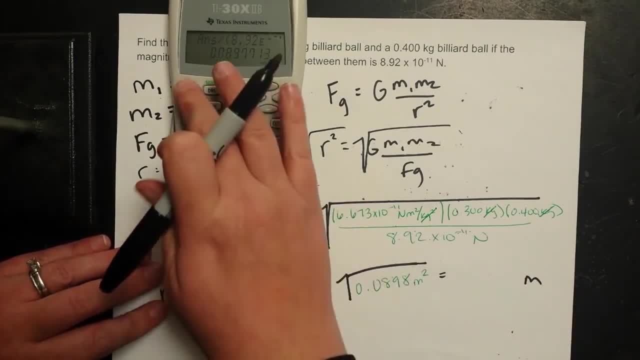 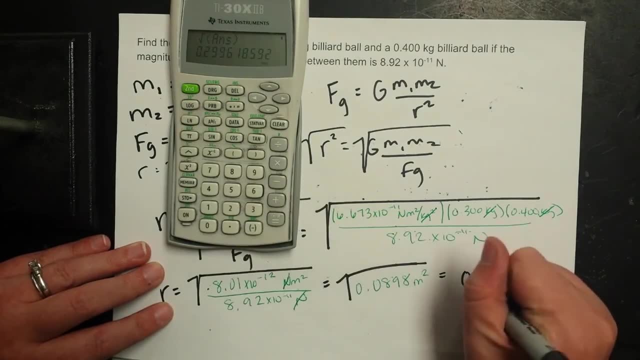 That makes sense for a distance. I'm going to take the square root of this value. Keep doing that. I've got chubby fingers today, So 0.3, because that's going to keep rounding up. So 0.3 meters. or another way we could do this is: